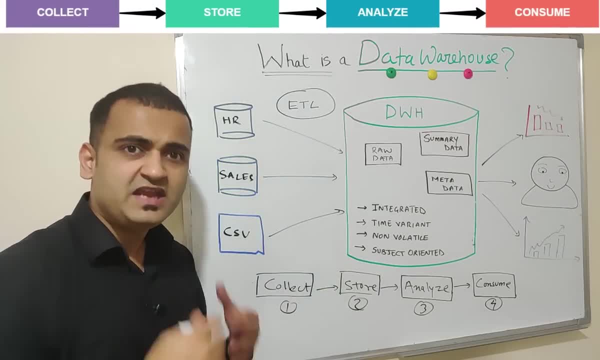 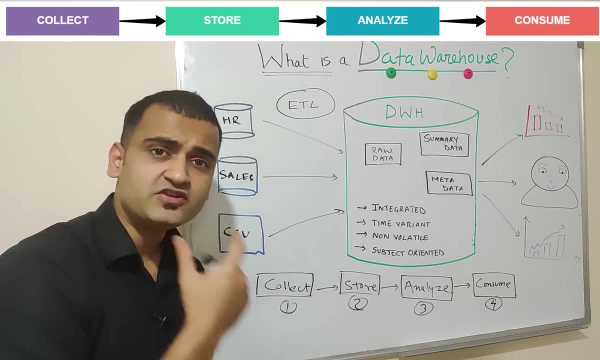 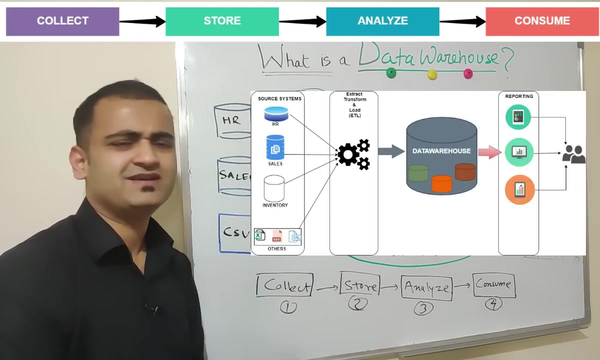 staging layer, and this process is done by the ETL process. what is an ETL process? ETL is extraction, transformation and loading of the data, and there are various tools to enable ETL for a data warehouse. you have Informatica, you have SAP Data Services, you have many others. so we are not discussing any product. we 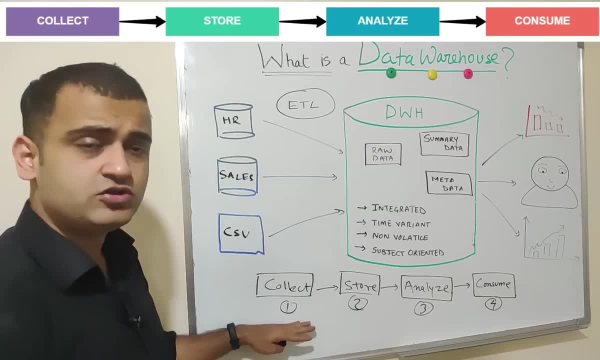 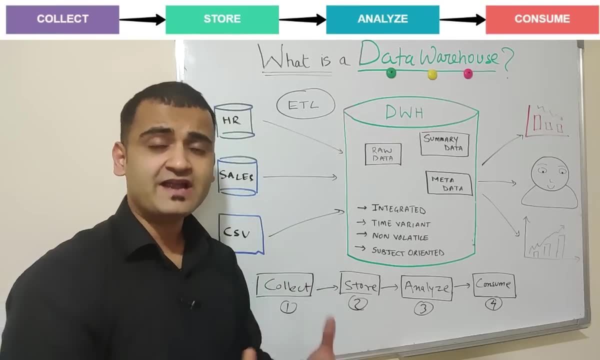 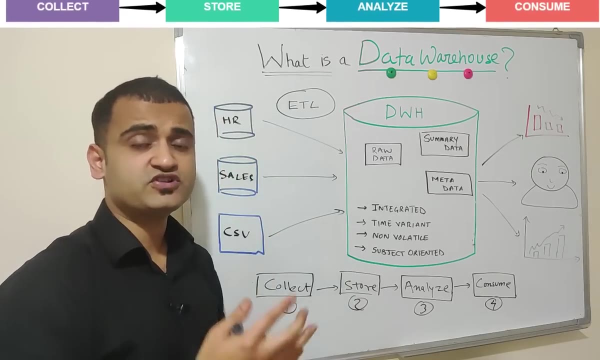 are discussing technology right now. so understand that first you collect the data in its raw form, store it somewhere in the second stage. then you analyze the data- what kind of insights you want from the data which has come in from the desperate systems in its raw form- and then you do those transformations to 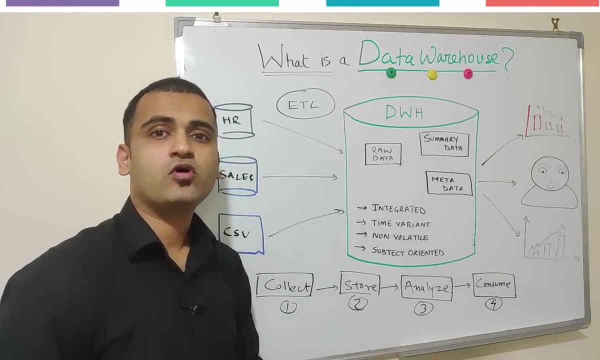 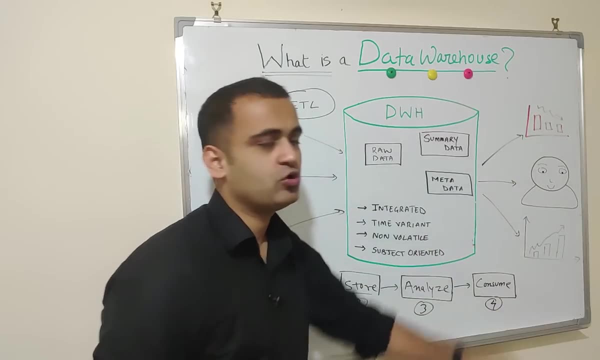 shape that data in a form, that data in a form where business can draw some kind of useful insights from it. and finally, at the consumer stage. it is the layer which you see at the right, where you see all these graphs. there are various tools like tableau, business objects you have. 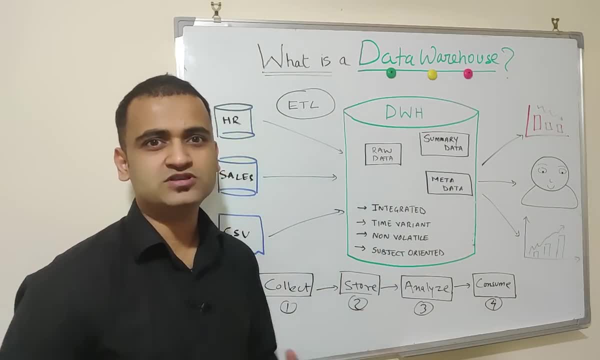 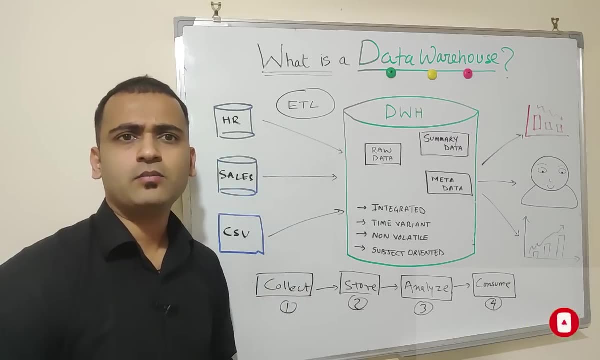 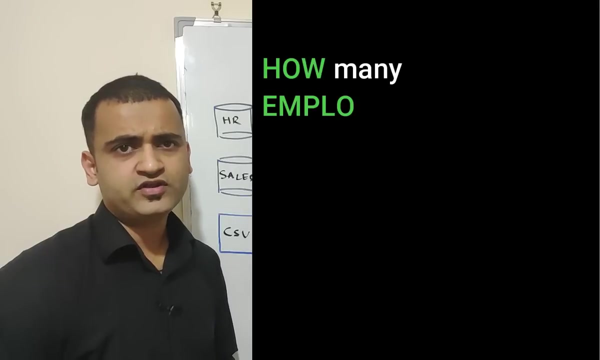 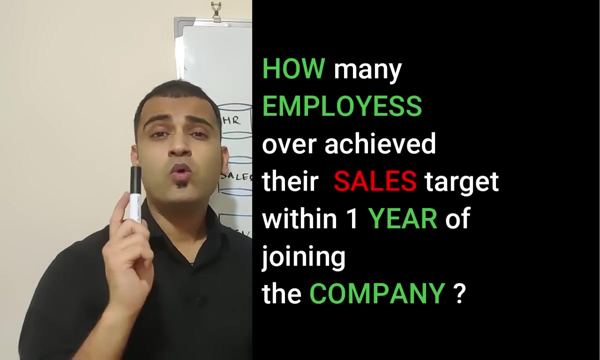 various tools to explore the data. so all these set of tools combined together make a whole data warehouse paradigm and a platform. so let's understand better with an example. suppose a company wants to analyze how many employees have exceeded or overachieved their sales target within one year of their 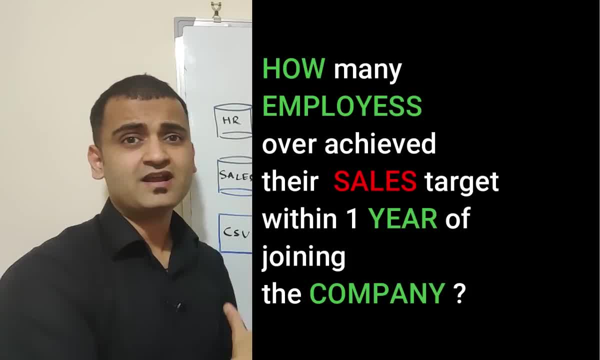 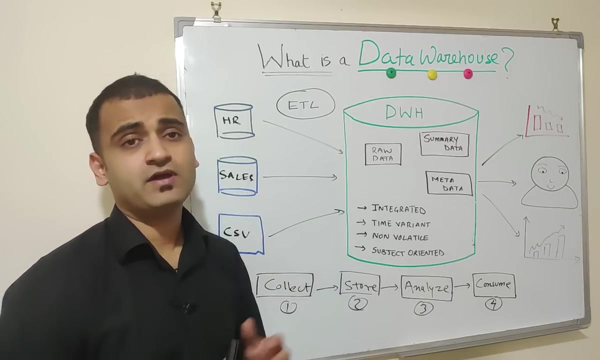 date of joining. now you can understand that there are different dimensions coming into picture. one could be the employee details, like employee name, employee ID and his or her date of joining, and second would be the sales which was generated by those employees in the sales system. now this information has to be analyzed and give and business has to analyze. 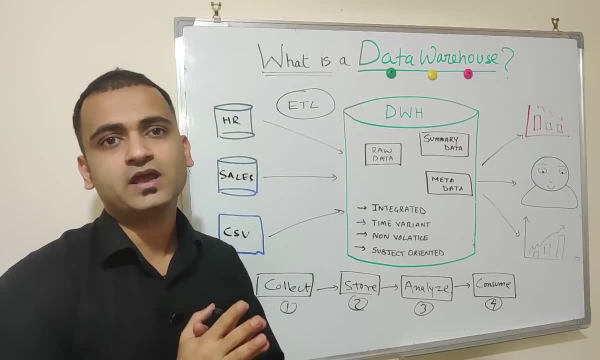 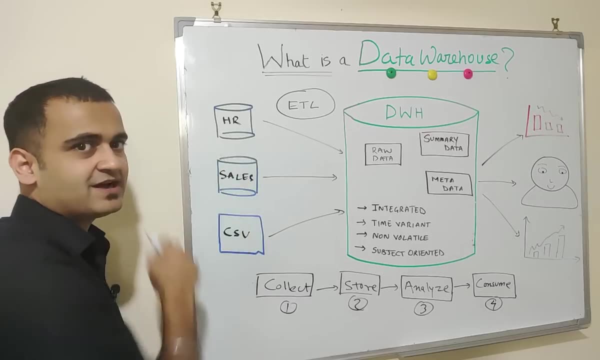 this information to understand who all are the best performing employees within the first year of their joining. so what you can do, you already have your HR system where you have all your employees data, and then you have your sales system, transactional system, where you have all the sales related information coming in. 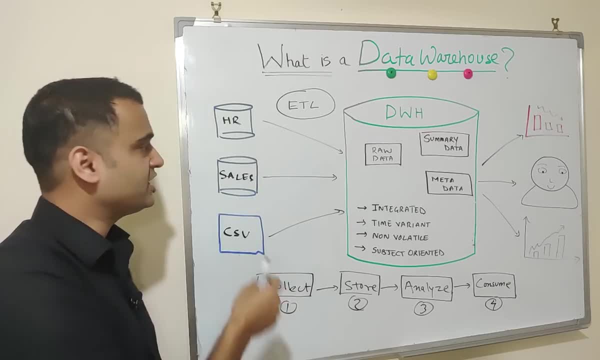 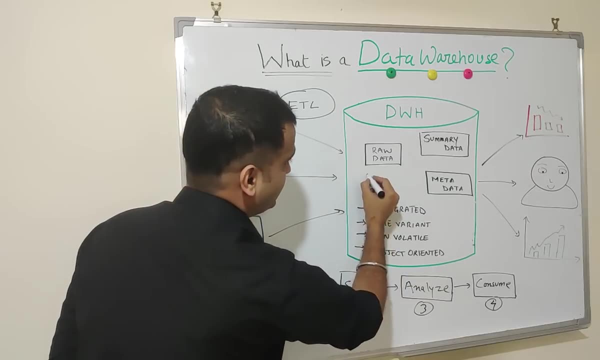 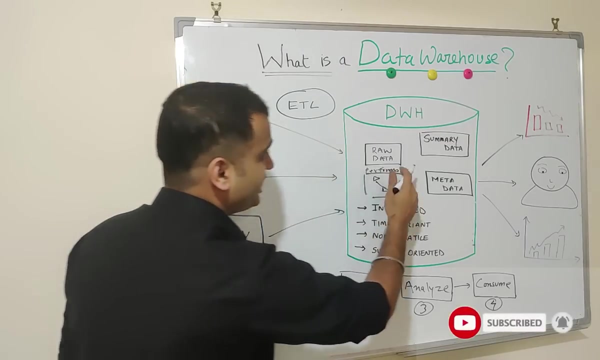 where you also have the information of the sales generated by each and every employee, so you can bring these two data sets into a data warehouse and create a performance, create a performance data set and in this data set you can combine all the desperate data coming from HR and sales to create a summary data which 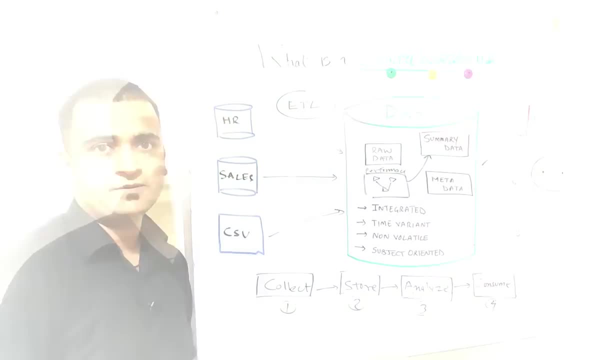 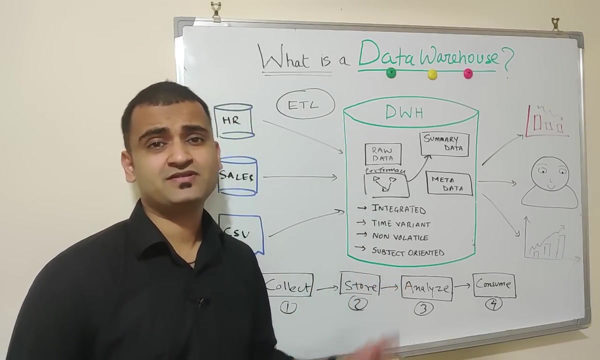 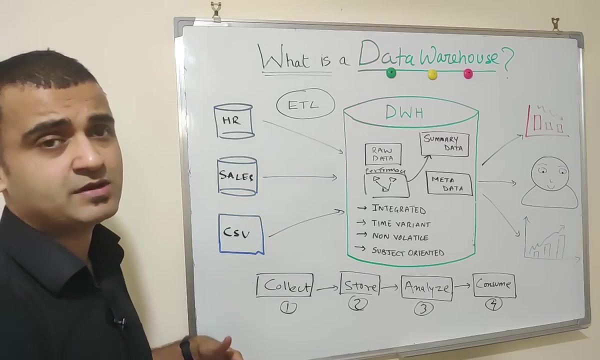 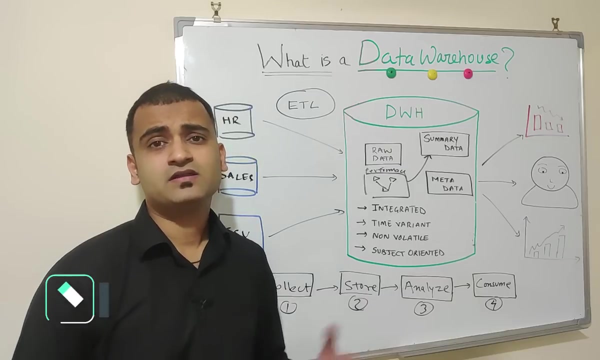 can be further distributed to the higher management. so now quickly understand some basic characteristics of a data warehouse. first, one is integrated, as the name suggests, integrated means data warehouse. enables you to integrate the data coming from various systems in a in a common format, and that helps you in further analysis. time variant: that means that 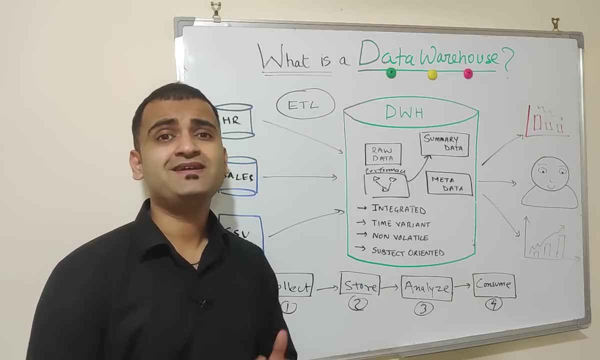 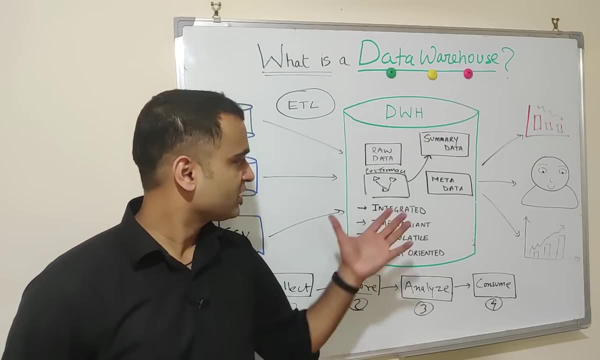 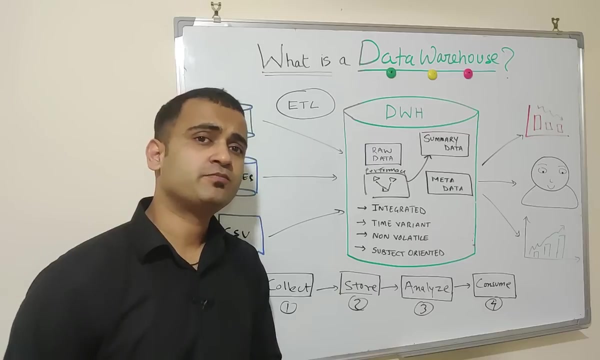 whatever data you store in the data warehouse varies with time. that means that you can do time study, you can do analysis based on time dimension, based on the data from various systems. suppose you want to do an analysis of your employees performance for the past ten years, so all that analysis can be done with the 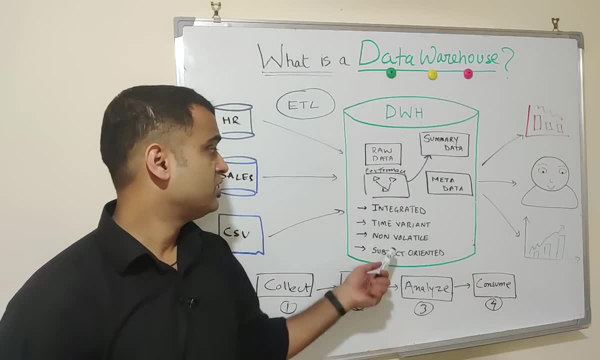 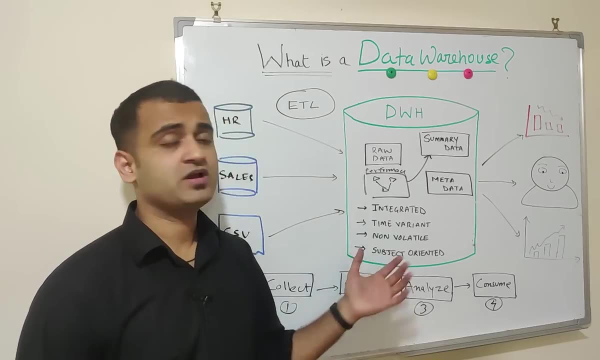 data accumulated and stored in a data warehouse. third is non volatile. non volatile means that whatever data comes in to a data warehouse remains static. it does not change. whenever you have a change, there is a separate mechanism to store that change into a data warehouse data warehouse. but once a data enters into a data warehouse, it stays there. 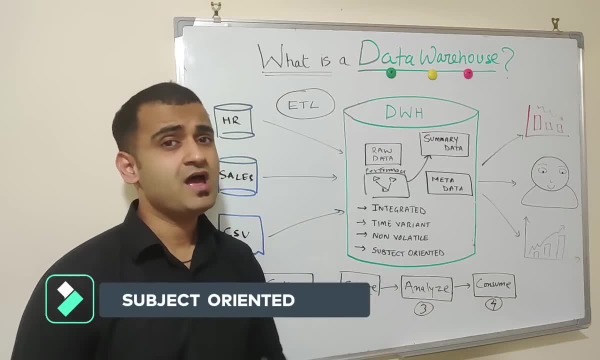 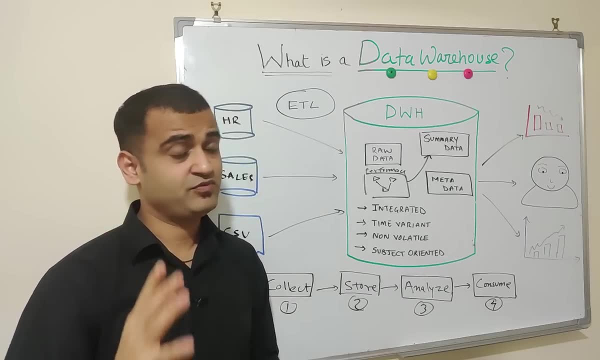 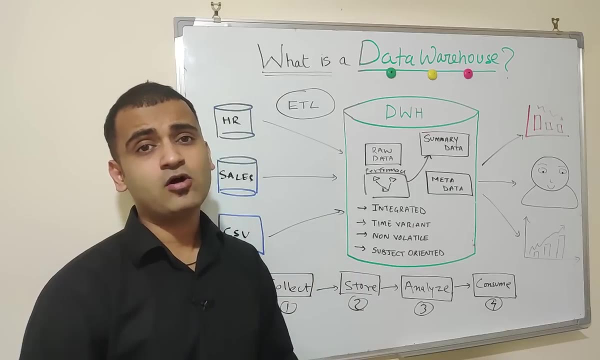 forever. and the last and the most important one is subject-oriented. understand this, guys: that data warehouse is built to serve specific purposes, and that is where it has to be subject-oriented. if you want to analyze something related to a specific area of interest, then you have to design your. 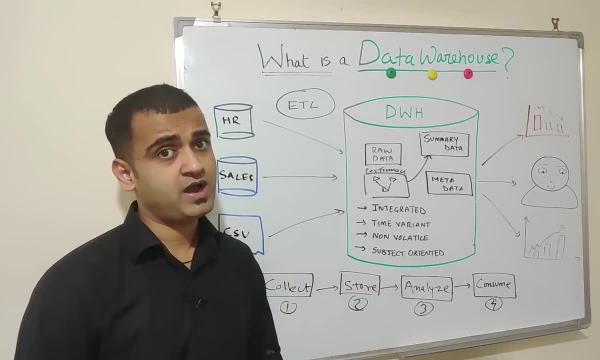 data warehouse. considering that subject into into the mind, suppose you want to analyze the overall sales of your company, then it would be more of a sales data warehouse and that's where it becomes quite subject-oriented. you have always need to understand that what you exactly want from your data warehouse. 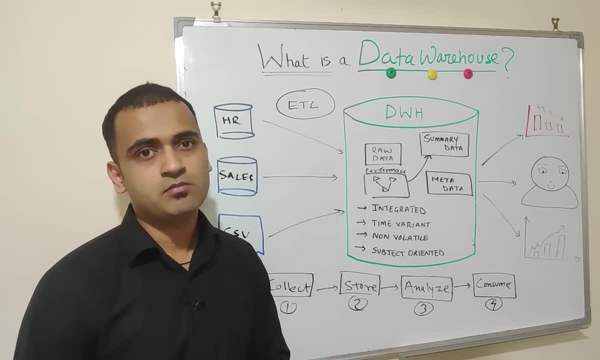 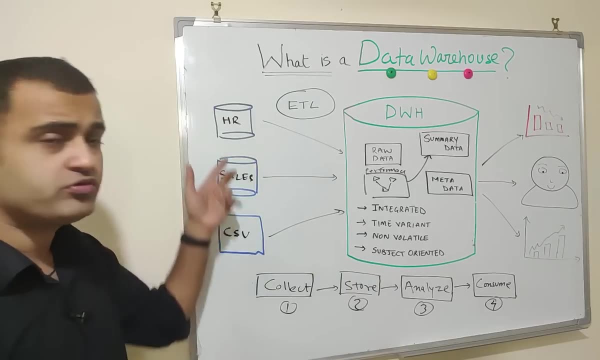 and then you design the data warehouse in that manner. let's quickly understand how a data warehouse different from a normal operational database, all your transactional systems, stores the data as in, as, as and when it is happening in the system, as it is happening in the system as and when it is happening in the 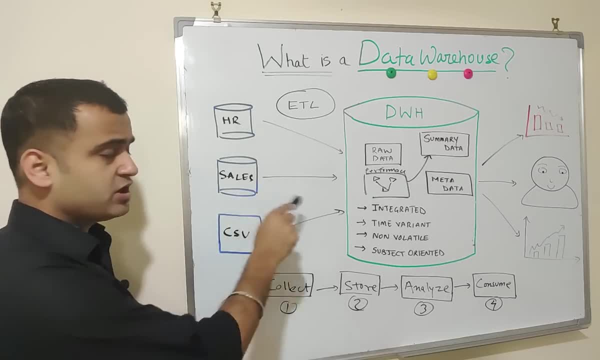 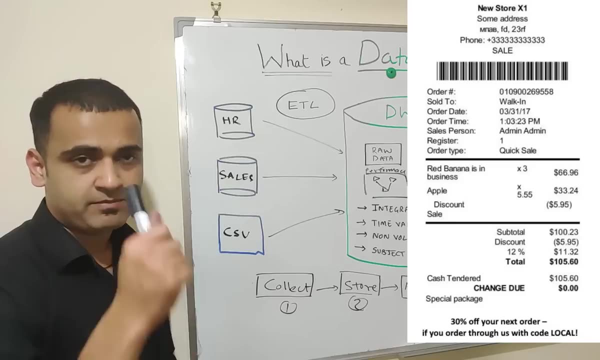 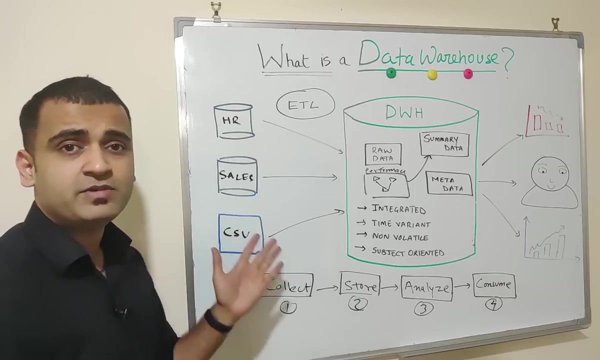 system as it is happening in the system. so suppose your sales database is recording all your sales transaction as and when any customer comes to the point of sales and makes a payment, then that transaction gets entered into your sales operational database. all these databases are made for faster writes because the 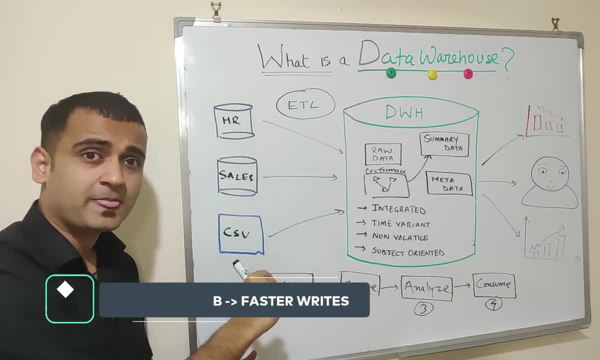 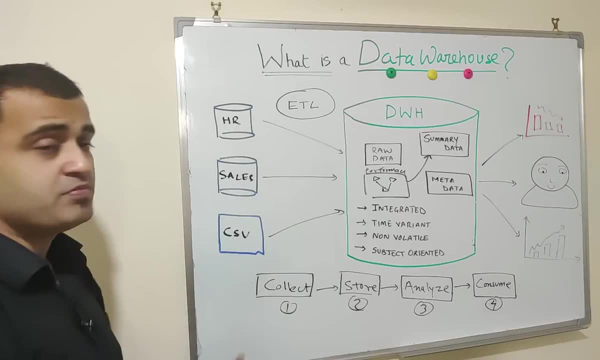 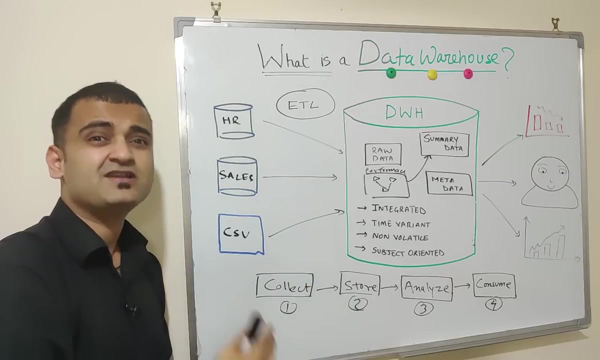 objective is to store the transaction as quickly as possible, but the same data then pushed into the data warehouse- and the objective of the data warehouse is of data warehouse is to make faster reads- because you are analyzing this data for not only one transaction. you might be analyzing this data for years and years of data accumulated. 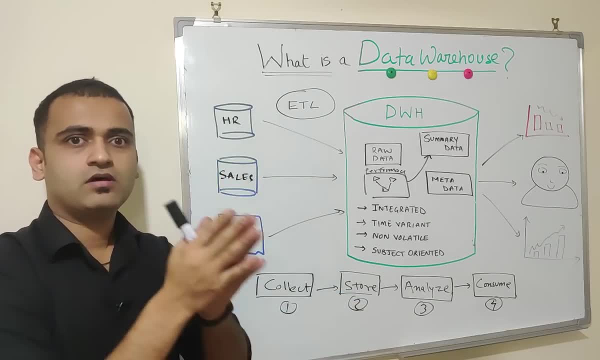 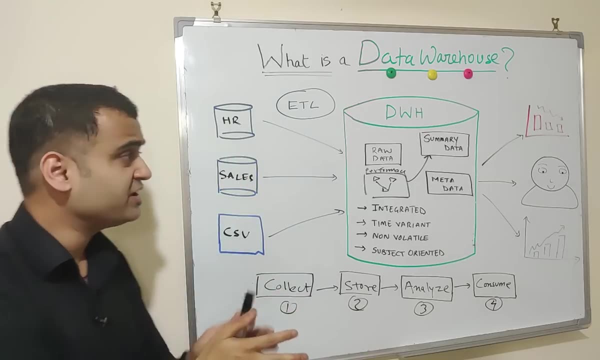 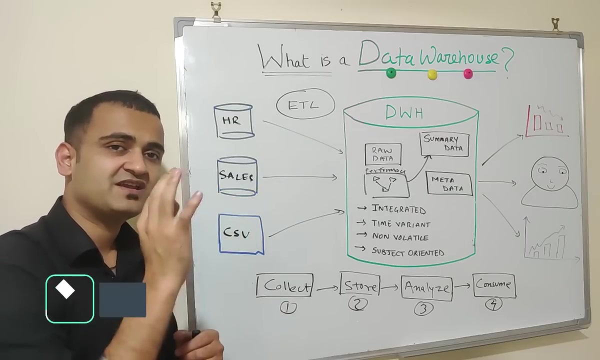 across various dimensions like country, geography, customer, employee, all these stuff. to understand your operational database, your OLTP database is different from your OLAP database, So your OLTP database stands for online transaction processing. the name suggests what I am trying. 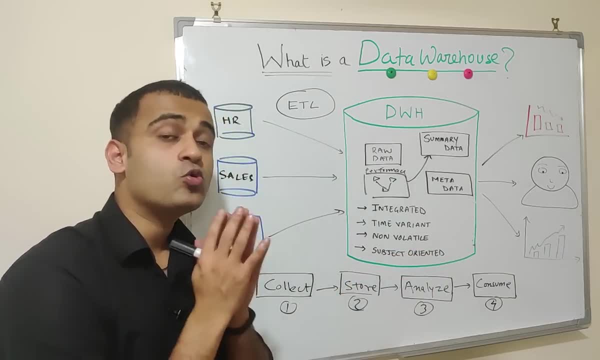 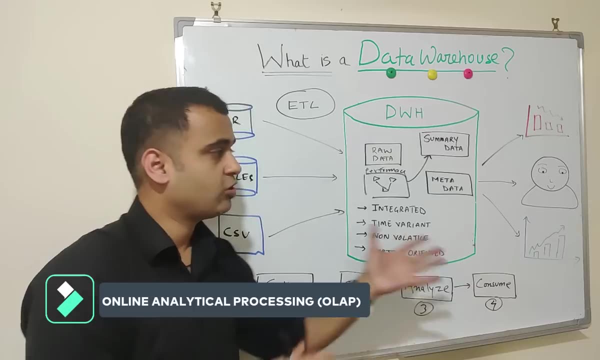 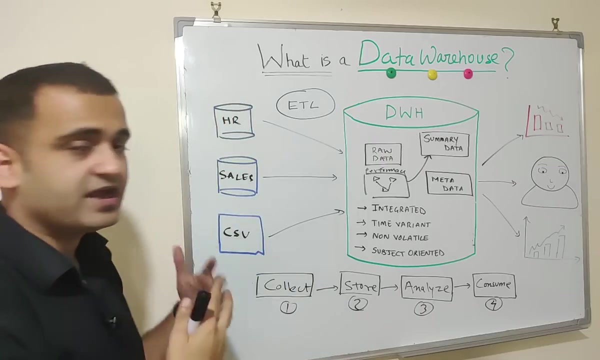 to convey here. In the same manner, your data warehouse is an OLAP database, which is online analytical processing. So understand, here we are doing the analysis of the data which is being fetched from your transactional systems. So this is a very high level understanding and differentiation between an operational 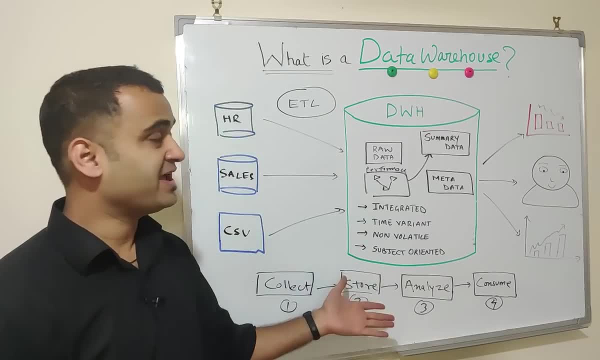 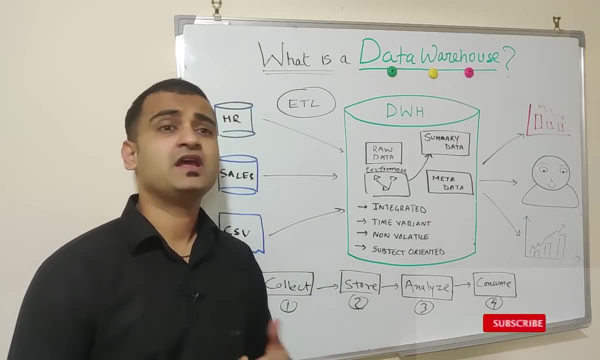 database and a data warehouse. So, guys, This is the very basic understanding of a data warehouse, but obviously, with the advent of new technologies and kind of data we are getting in various formats: structured, unstructured, streaming data, batch data. there are various data warehouse designs which are coming into. 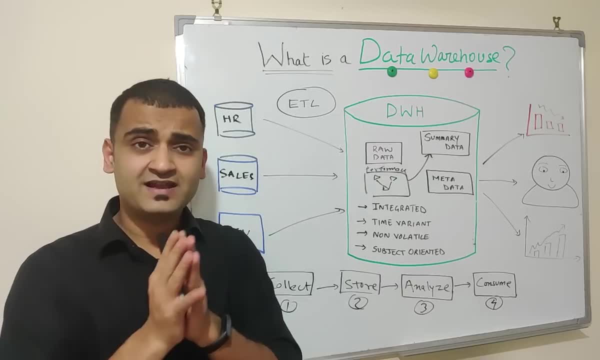 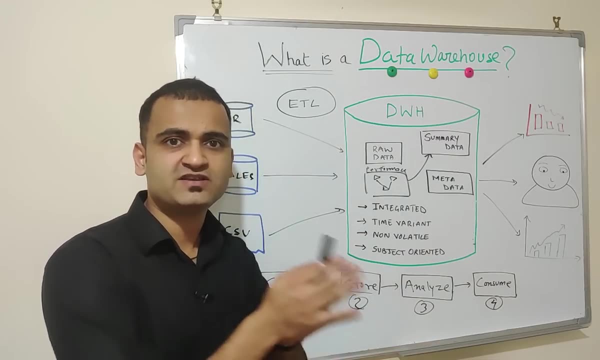 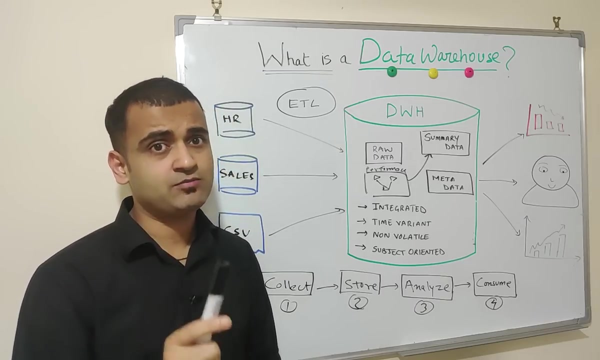 the picture. now. There are technologies like data vault, data lake and, in tandem with data marts, which can be used to provide solution to a specific business case. and yes, if you want to understand data lake and data vault, I have very good videos made on the same topic. 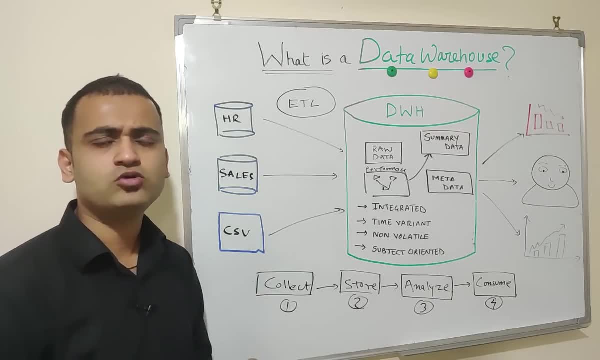 So take, for example: you want to analyze data coming from your Twitter handle to identify and perform some sort of a sentiment analysis. So all that kind of data is unstructured data. So that's where you can put a data lake in between and that data lake can contain all. 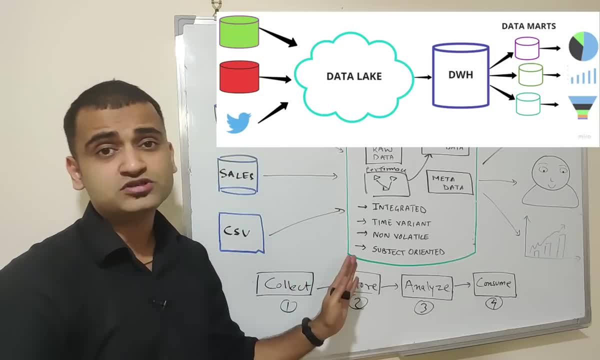 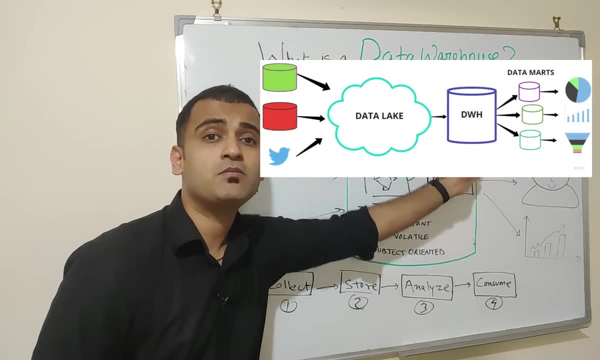 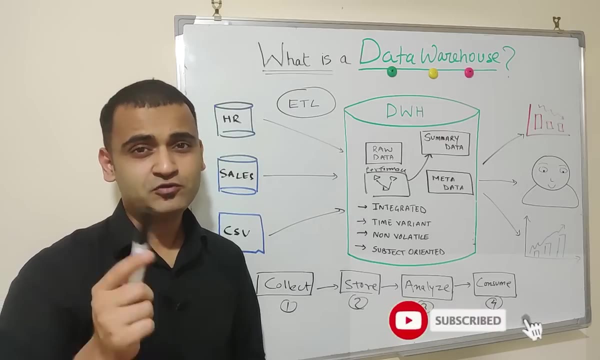 kinds of data coming from all kinds of sources, then push that data into a data warehouse and even to further optimize that, You can make further specific data marts which can be finally consumed by the specific business area. So I hope you liked the video. 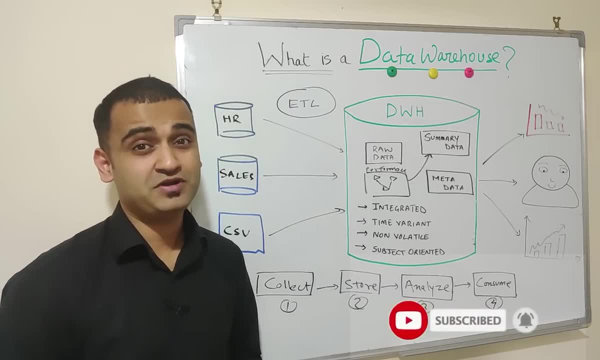 If you did consider subscribing and hit the bell icon for more updates and also give a thumbs up so that YouTube understands that there is some worth in this video which can be shared with others. Thank you so much and keep hustling. Bye for now.